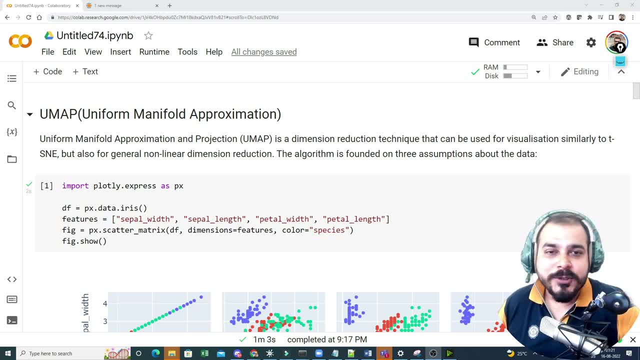 you can use UMAP to reduce the number of dimensions, but this is far more superior than PCA or TSNE. Why I'm saying you? I'll show you a practical example right now And we'll try to see that- how UMAP can be used to basically visualize higher dimensions. In short, when we reduce this into 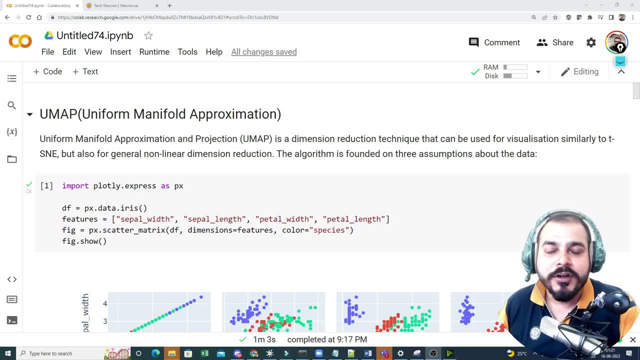 some smaller n number of dimensions at that point of time, like suppose, if I reduce it to two dimension or three dimension, the amount of information that is lost is a little bit less when compared to PCA or TSNE. And again, there is an amazing research paper regarding this. You. should definitely have it. So if you have a PCA or TSNE, you can use UMAP to reduce the number of dimensions. Why I'm saying you? I'll show you a practical example right now And we'll try to see that how. 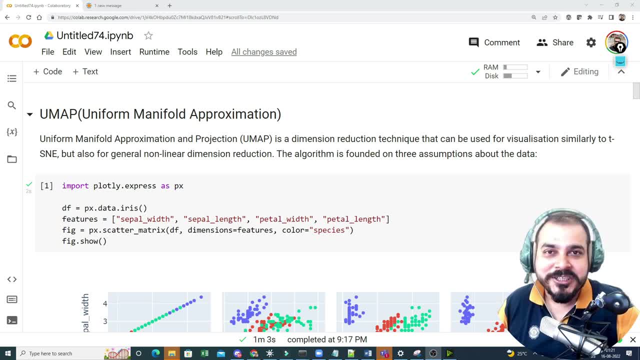 UMAP can be used to basically visualize higher dimensions at that point of time And we'll try to have a look on to that. If you probably want the theoretical explanation, make sure that you hit the like button. at least make it to 500.. I'll definitely upload the theoretical explanation. 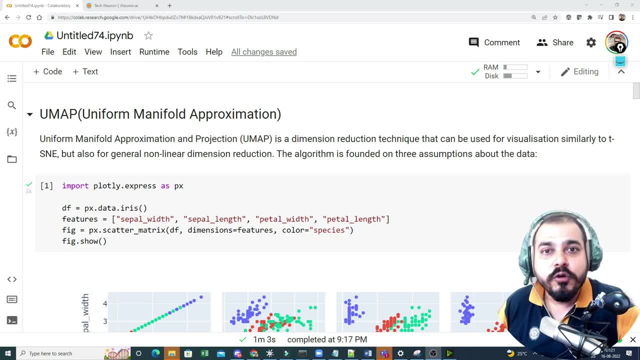 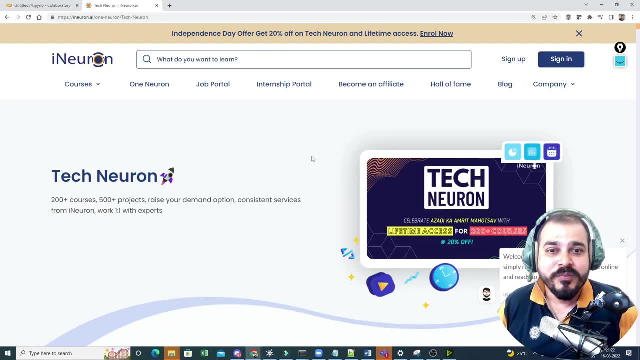 about UMAP, But today, in this video, I really want to show you how UMAP actually works. Now, before we go ahead, there's a quick announcement regarding the TechNeuron offered by iNeuron. So in TechNeuron, if you don't know, it is an OTT platform with 200 plus. 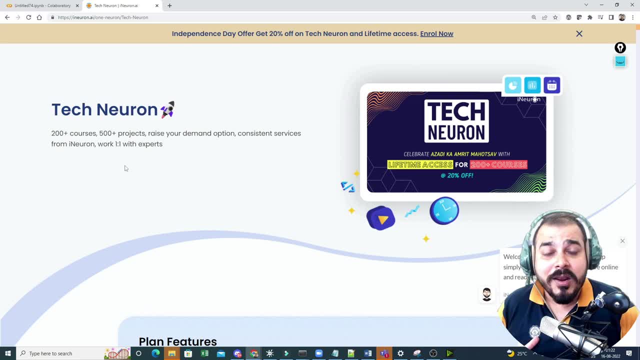 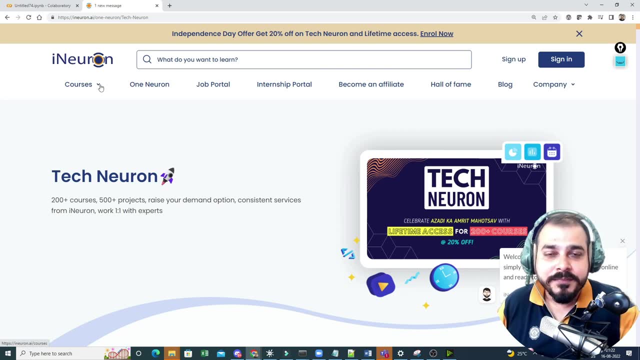 courses. Currently it has 240 courses And along with this, you know, you also have a all the live classes that is included. So live batches, whichever we run in every month. that will also be included in TechNeuron And currently we are launching the lifetime offer. 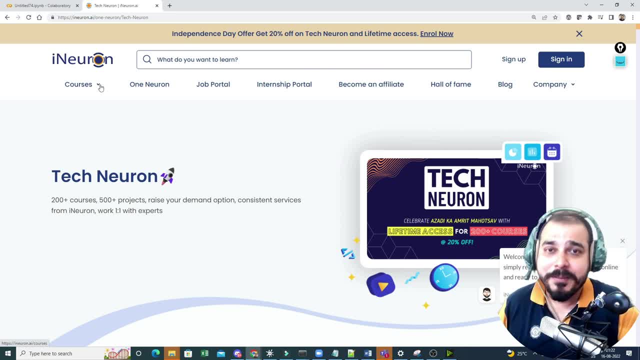 which will be for a week. This is just for the. on the eve of Independence Day, we really wanted to help many people out who are not able to afford other courses, So through this they will be able to get all the other courses, along with that, all the live sessions, also The price of the course. 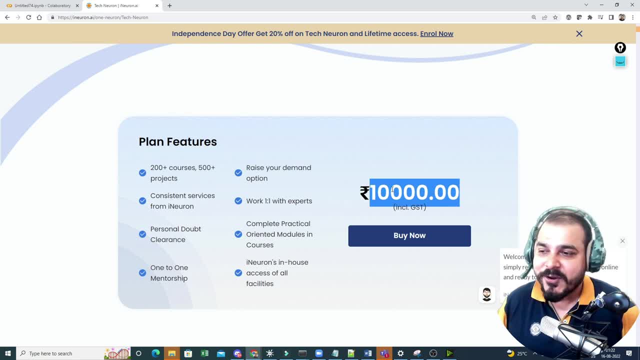 has also been reduced to 10,000 rupees, And if you're not satisfied just with 10,000, what you can do is that you can use a coupon code that is CRUSH20.. And then you'll be getting a 20% discount. 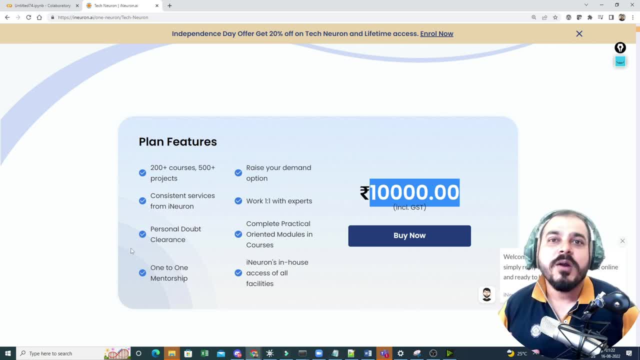 So in 8,000 rupees, all these courses along with many services, seven days. you'll be having a doubt clearing session. you'll be having one to one mentorship. you'll be having probably mock interviews, resume discussion. you can also raise a request with respect to any kind of courses that. 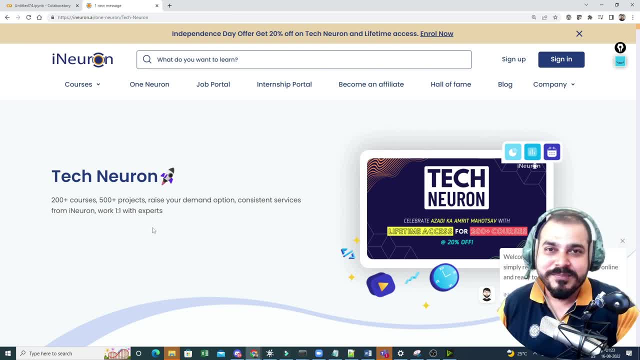 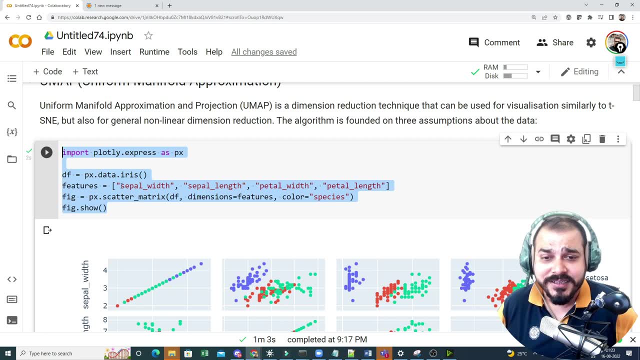 you're interested in. So the offer just is for another four to five days. please utilize this opportunity. Okay, now let me go back over here. Now, over here, I have first of all taken an Irish dataset. Here you can see sepal width, sepal length, petal width, petal length, And I've just 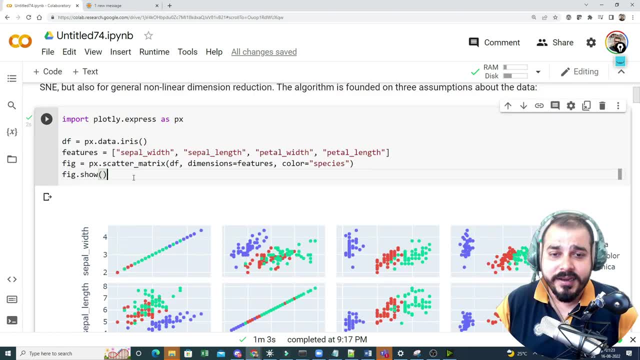 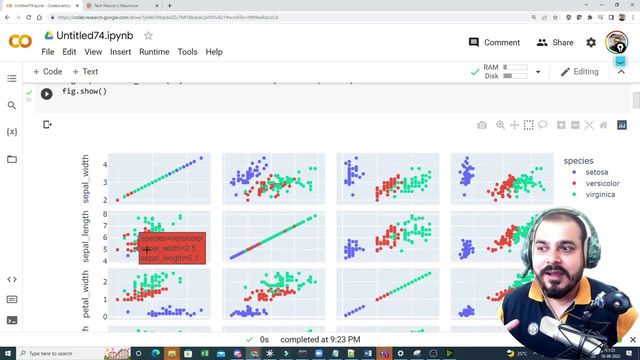 created a scatter matrix, And here you can see how my diagram is basically generated, Right? So this is what is the plot that you can see, And obviously this is not like. this is just like a two dimensional plot, Right? with respect to different, different features. you can do the similar task with the help of: 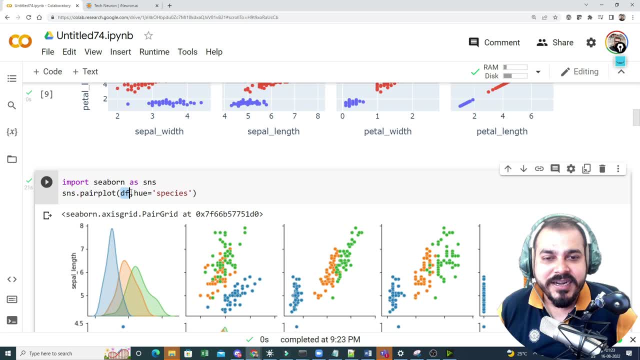 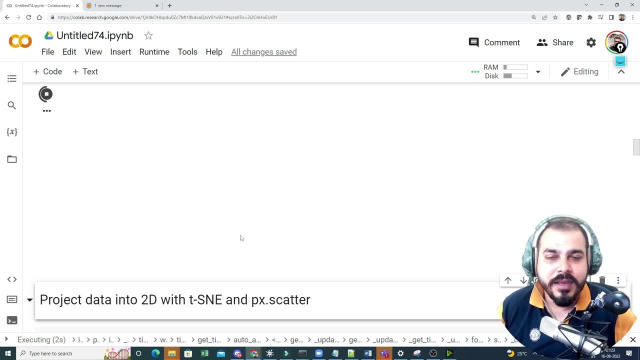 Seaborn, where you just need to write snhpairplot with the entire DF And here you can just try it- who as the species so that it can actually categorize. So once you execute this here, you'll be able to see that you'll be getting a pair plot wherein it will try to show you the correlation. 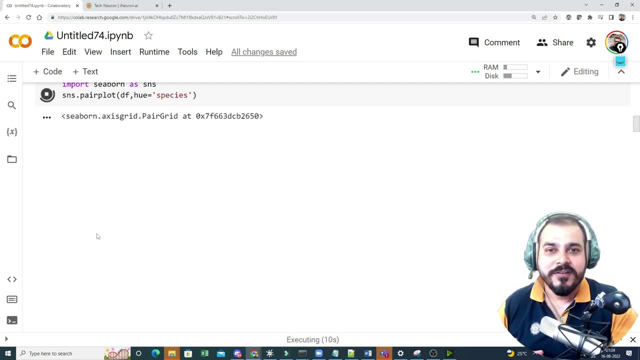 between each and every features, right, specifically independent features. that is what we are actually focusing on right now. Now, as you know, this will probably take some amount of time, So here I'm going to show you how to do this. So let's go ahead and start. So let's go ahead and start. So here I'm going to show you how to do this. So let's go ahead and start. So here I'm going to show you how to do this. So here I'm going to show you how to do this. So here I'm going to show you how to do this. So here you can see that your graph is ready. 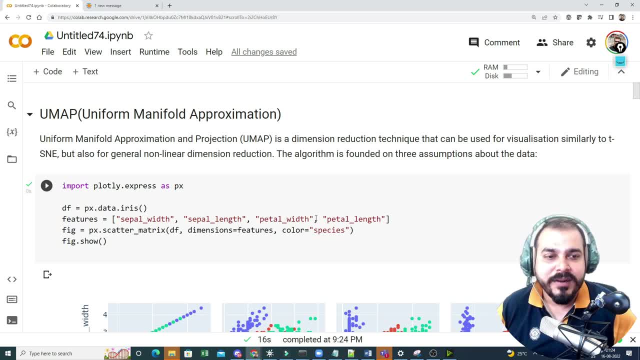 here I'm going to show you how to do this. So here you can see that your graph is ready Now. already you know that we have four features: sepal width, sepal length, petal width, petal length- right, So four dimension. Now let's see when we 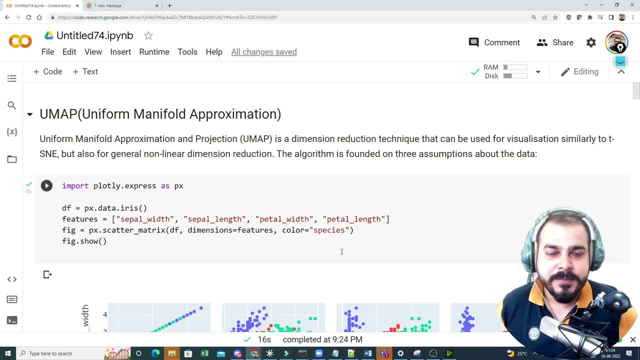 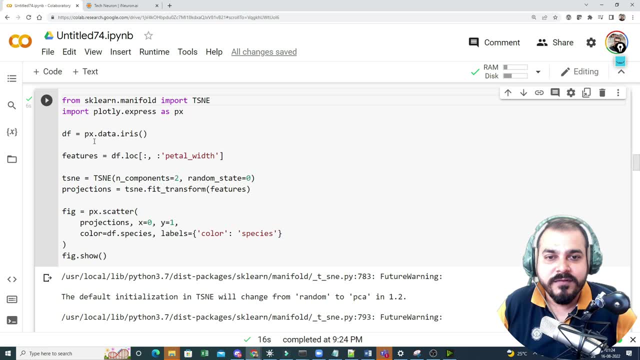 reduce this number of dimension into two with the help of t sn e, how my data will look like. So here it is. project the data into 2d with t sn e. So here I have taken all my features, and then I'm just using t sn e, And when I 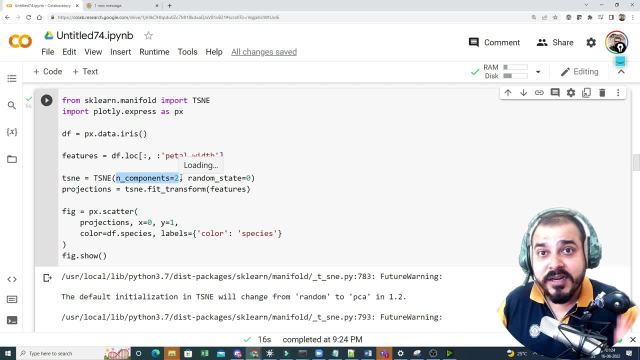 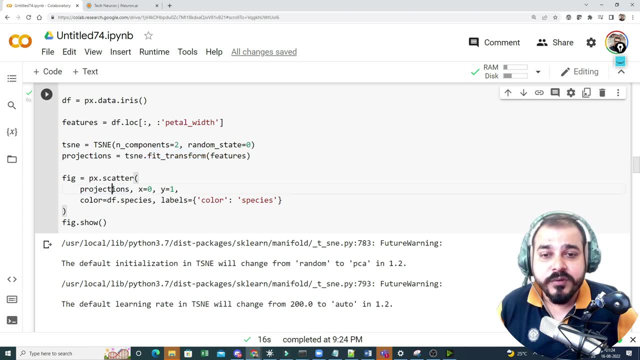 write n underscore components is equal to two. that basically means I'm converting that four dimension into two dimension, And then I do fit transform on the feature And then I'm plotting the scattered plot with respect to all these projections and my x and y value, right, And here you can see, I'm also provided my labels, along with the color that I 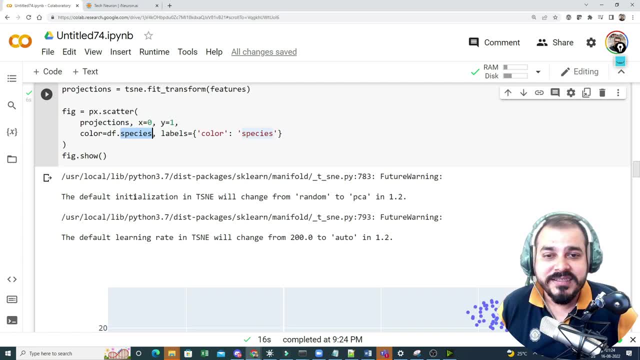 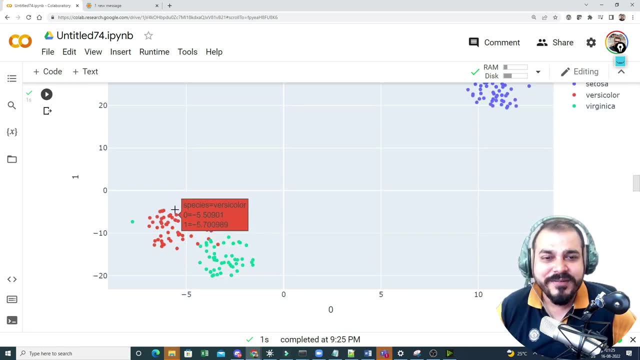 really want to specify with respect to my output feature. So once I probably execute this, let's see how we will be able to see it. And here is how clearly we can see. fine we have. we have reduced this number of dimensions into two right. 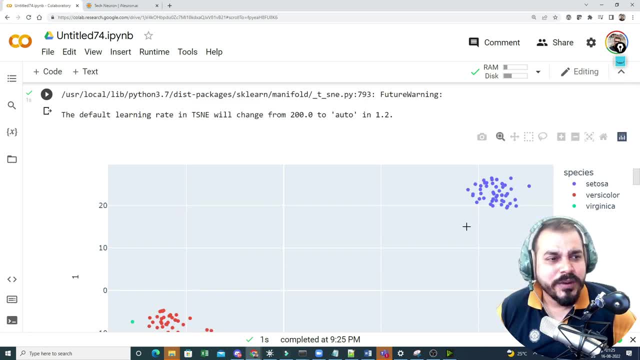 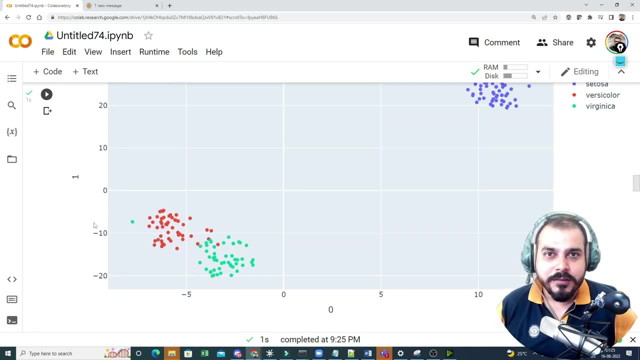 all the four features And here here, by seeing this, yes, you can clearly separate it, but what if I make or project this into three dimensions? Okay, And obviously, if you have many number of features, then again some amount of information is definitely lost. 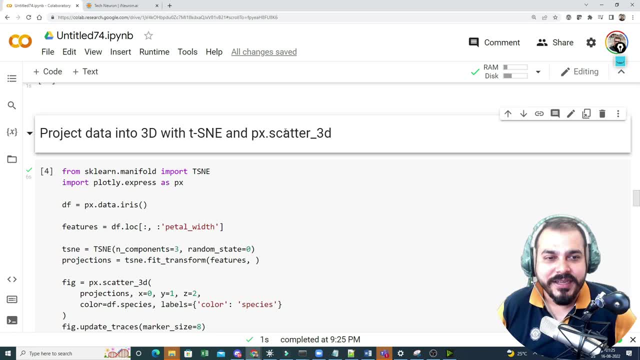 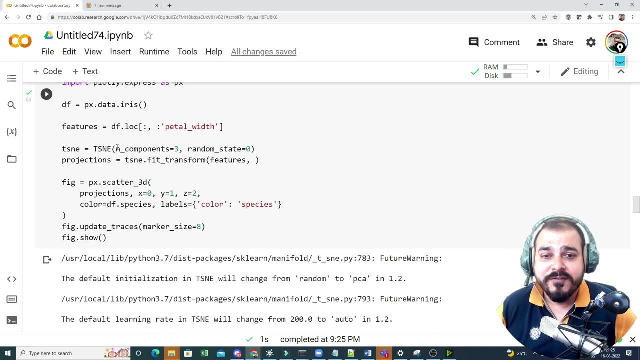 Now let's go ahead and see projecting the data into three: d with t, sn, e, right, the same technique, that is, dimensionality reduction technique. Here you can also use PCM. So here what I'm doing, I have taken n underscore components as three. 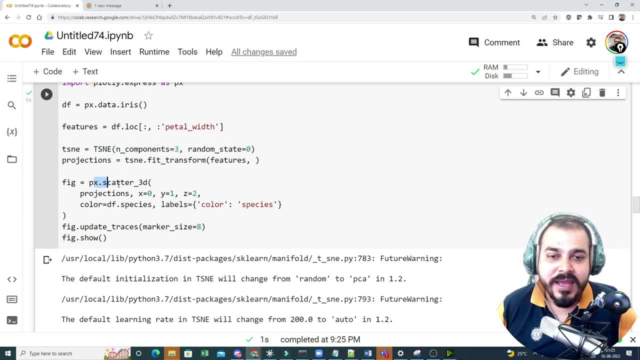 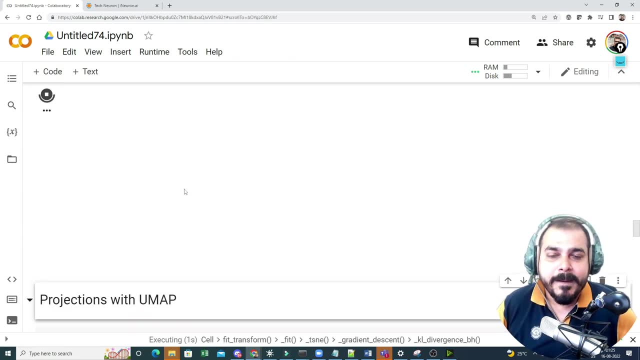 that basically means that is going to convert this into three dimensions, and that is a reason reason why I've used scatter underscore 3d plot. okay, so once I execute it and here you'll be able to see this, here, obviously you'll be getting a three dimension. so this is how it looks like now. 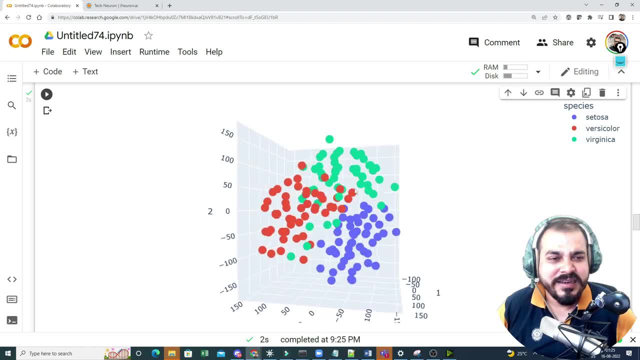 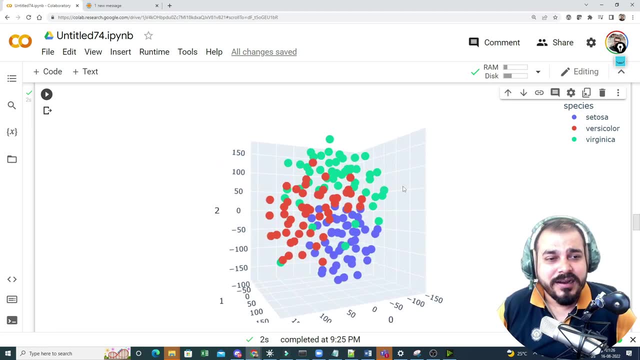 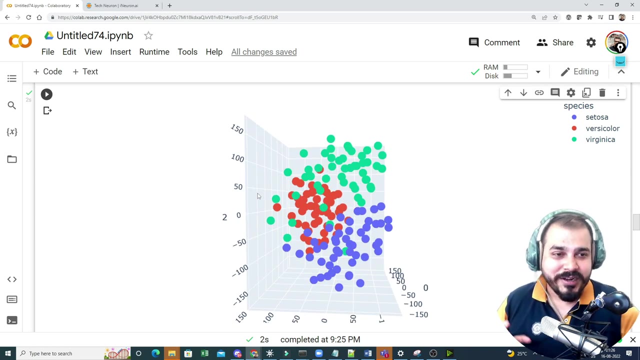 here. you can see that. okay, fine, my data points are completely jumbled right like: yes, there are a lot of overlapping. still, we are not able to properly see this entire dimensions. you know they are still overlapped data points and, yes, it is not that good when compared to what we really want. I really 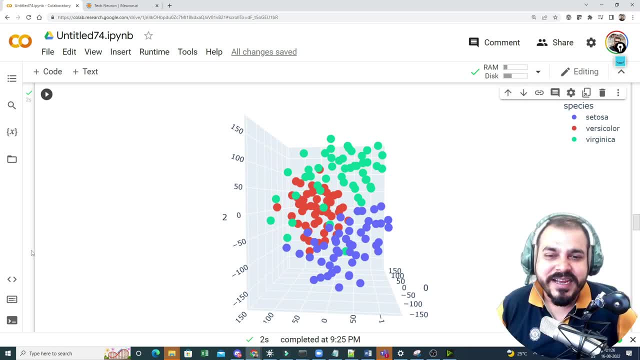 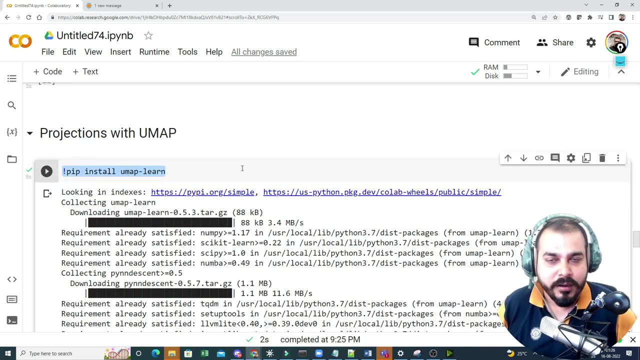 want this clusters to be completely separate. now let's see this technique with the help of UMAP. okay, so first of all, to start with UMAP, you have to install slash pip, install UMAP, learn so. once you install this, the installation will happen. I have already installed it. then all you have to do 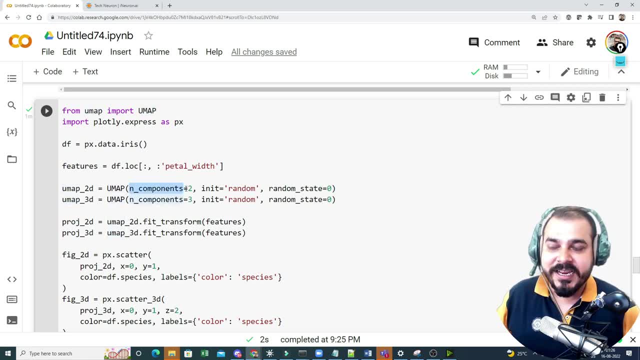 is that apply UMAP and again, it is an efficient technique when compared to PCA and TSNE. and if I give an underscore, components is equal to 2. that basically is it going to convert into two dimension, and then I'm also made sure that I convert this into three dimensions. so UMAP 2d. 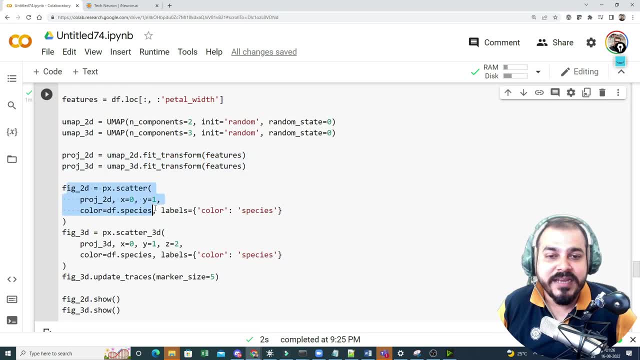 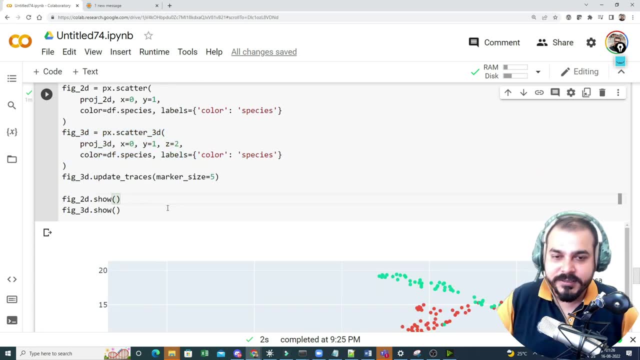 UMAP 3d, I do fit transform on the specific feature and I'm scat. I'm just creating a scattered plot with respect to the two dimension and with respect to the three dimension, and once I see this, you will be able to see how beautiful diagram I'm able to get with respect to two dimension, right over. 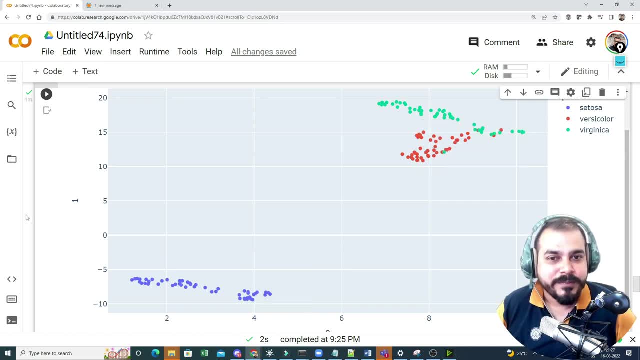 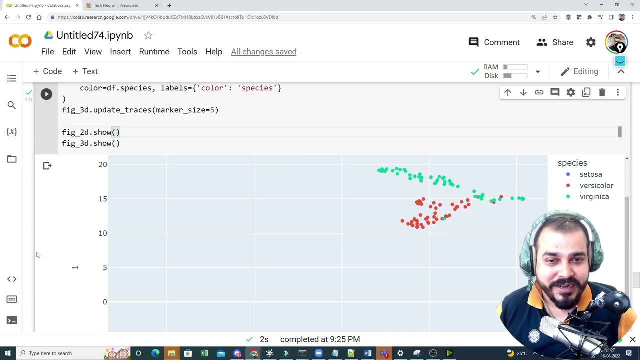 here all the data points are clearly separable with respect to two dimension. but the most interesting thing, what we saw over here with respect to three dimension. now you see, with respect to three dimension, the magic is here. now see this: how well your data points are clearly.